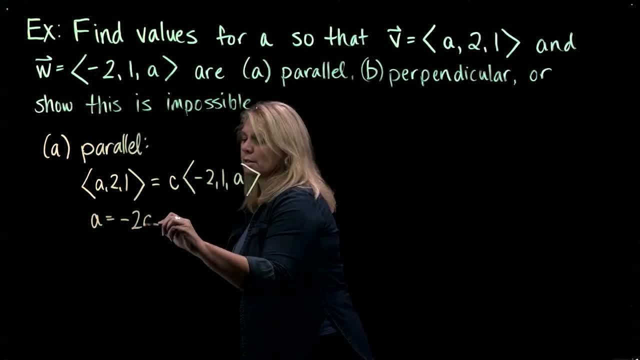 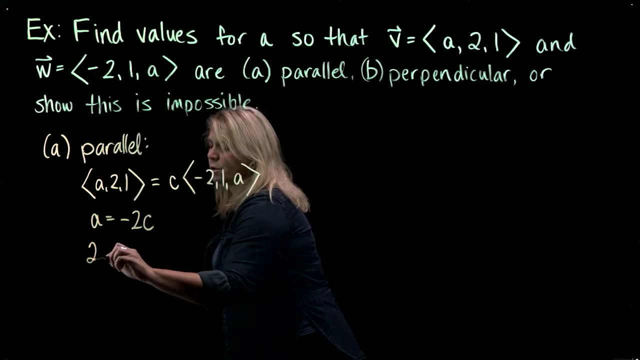 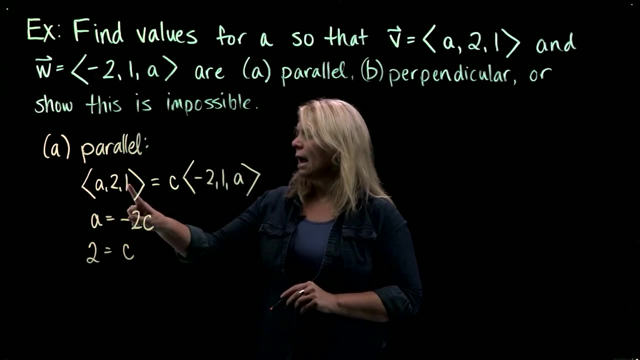 So I would have a equals negative 2c, And then the second components for this vector, and this vector would have to be equal to each other, so I would have 2 equals 1 times c, so c. And then the third component, I would have 1 equals and then over here I would have a c. 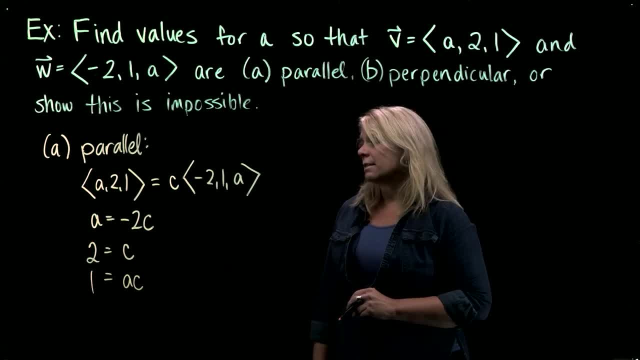 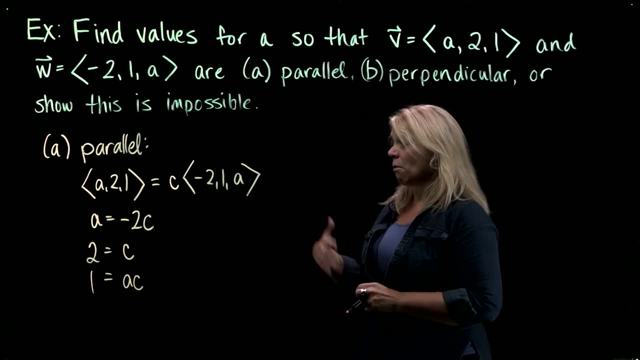 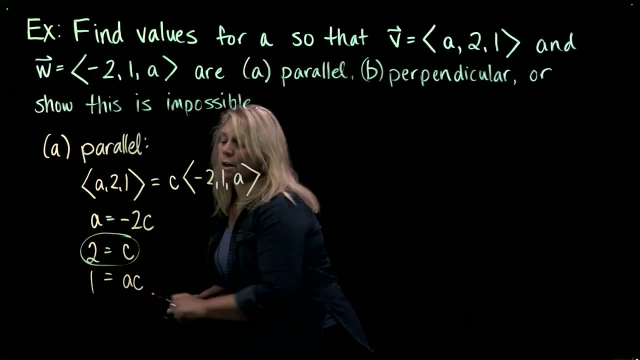 So I've just set the components equal to each other. What I have here is a system of three equations and two unknowns, so I need to solve that system and think about whether that system actually has a solution In this particular problem. the second equation here just gives us a value for c, so once I have that, I could plug that in. 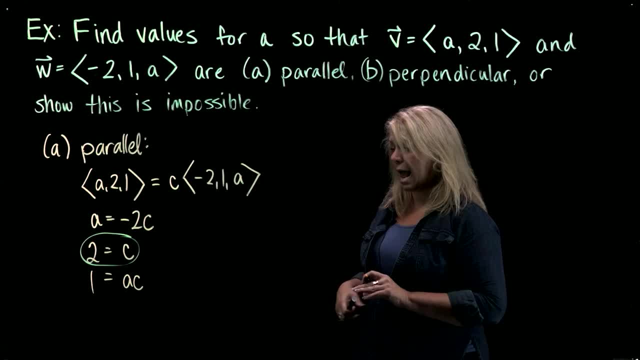 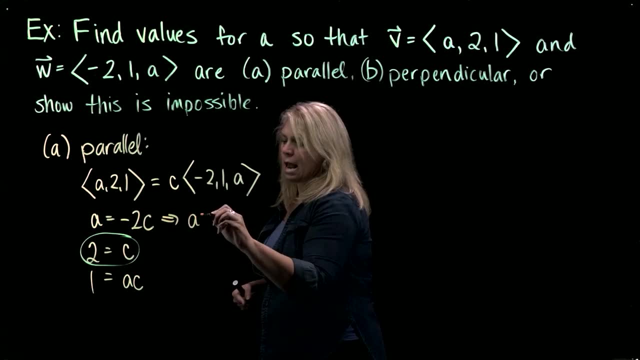 Either place and figure out a corresponding value for a. so if c equals 2,, then this first equation says that a has to equal negative 2 times 2,, so negative 4.. All right, so the second equation gave me c equals 2,. the first equation then gave me a equals 4.. 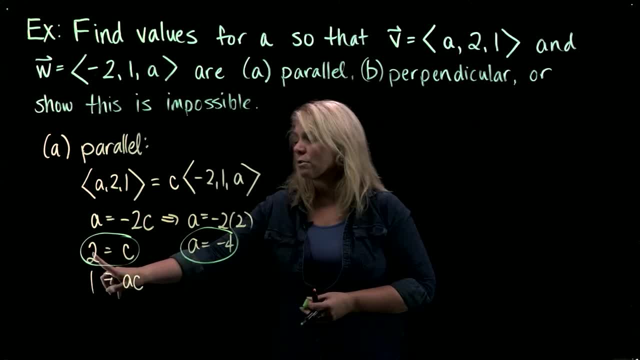 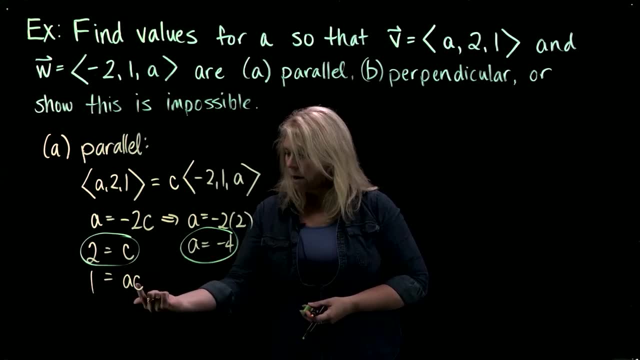 In order for this system to be true, I would have to check that those two values also work in the third equation. You'll notice that they don't. so 2 times negative 4, a times c is not 1, so these don't check. 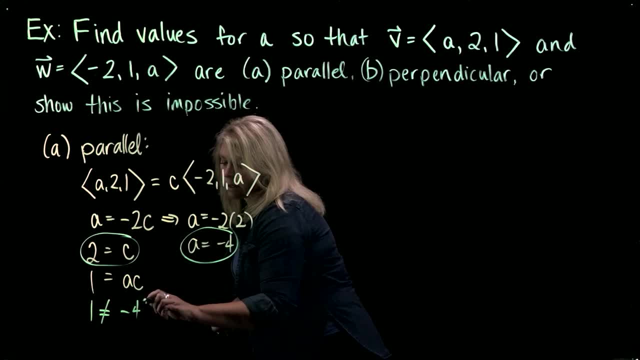 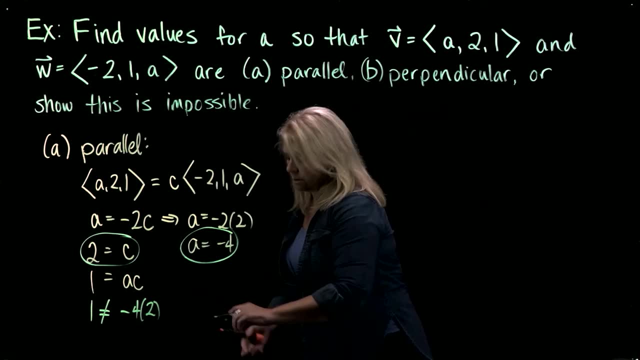 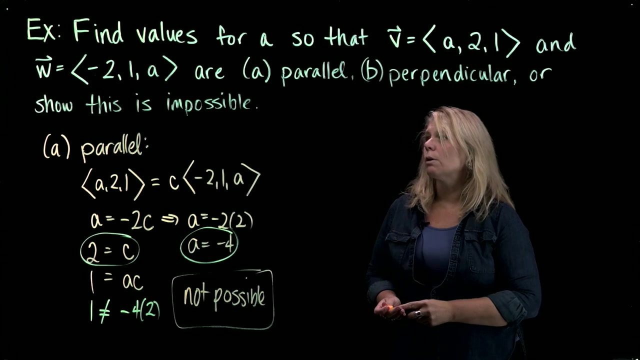 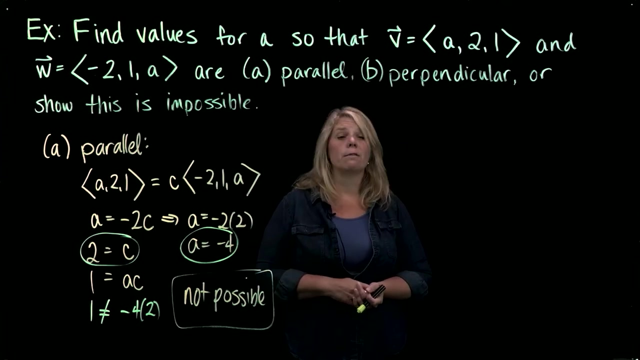 1 is not equal to negative 4 times 2, so those don't check. So in this case this particular part of the problem is not possible. All right, let's go on to the second part of the problem. here Again, think about if these two vectors were going to be perpendicular to each other, how I might think about finding a possible value, or show that it's impossible that the two vectors are perpendicular to each other. 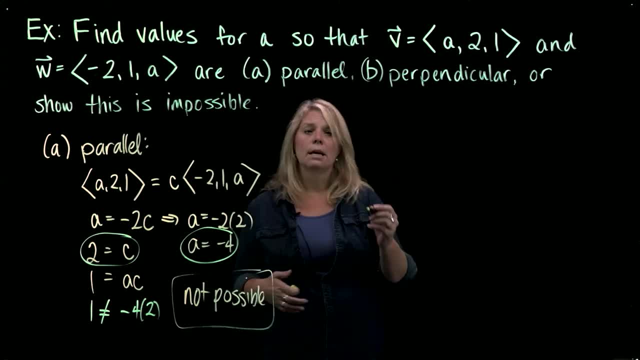 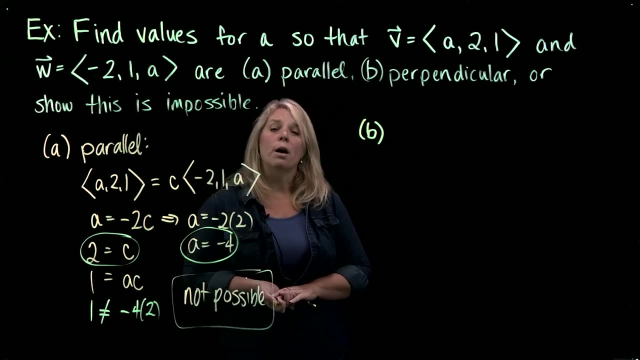 So again, I'm going to use an equation to think about this. So perpendicular vectors: that should make you think about dot products. One of the things we talked about with dot products is that two vectors are said to be orthogonal if their dot product is 0,. 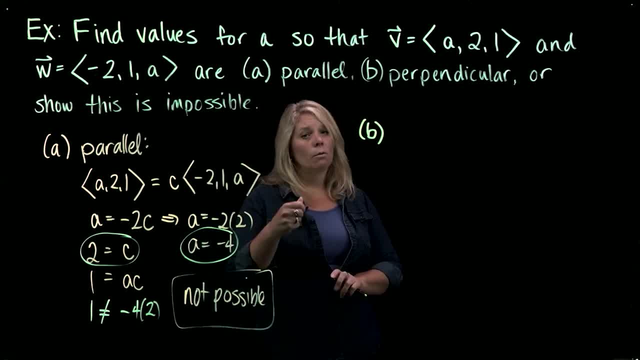 and that there are three ways that can happen if that dot product is 0. One of them is that one of the vectors is the 0 vector. The second way is that the other vector is the 0 vector. The third way is that they are perpendicular to each other.